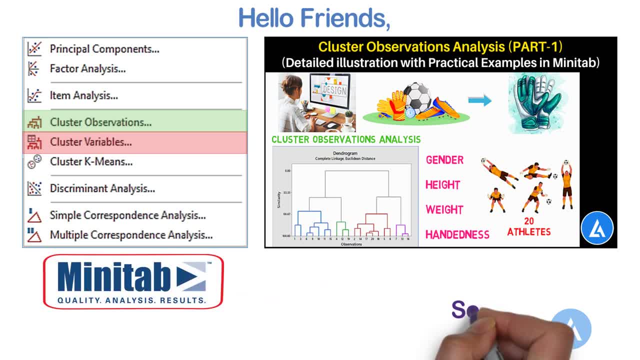 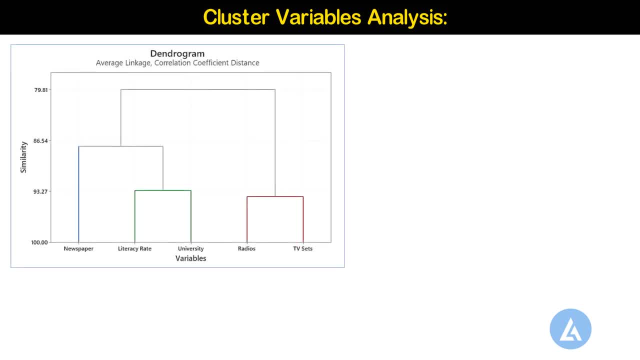 for easy understanding and better clarity. So let's begin. Cluster variables analysis. The cluster variables analysis is used to group variables into clusters that share common characteristics. Clustering variables allows you to reduce the number of variables for analysis. Similar to cluster observations, this analysis is also appropriate. 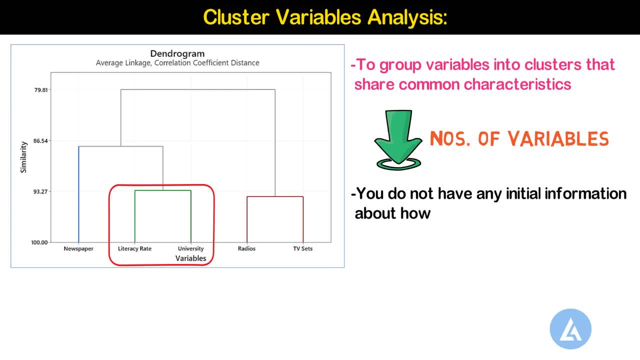 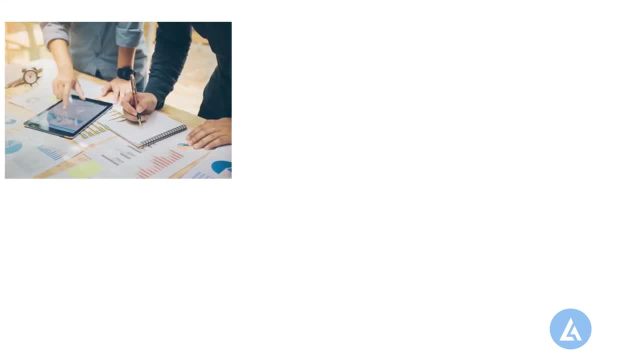 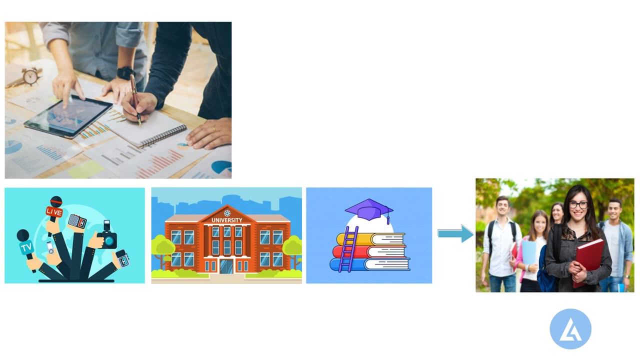 when you do not have any initial information about how to form the groups. For example, a social scientist wants to study the effects of the number of media outlets, universities and the literacy rate on the college admissions of the population For 10 cities around the world. the scientist determines the number of newspaper copies. 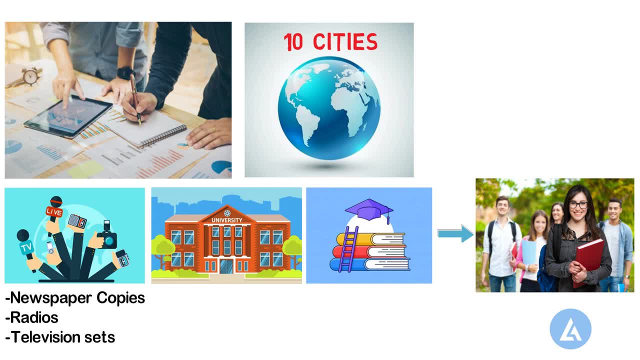 radios and television sets per 1,000 people. The scientist also records the literacy rate and whether a university is in each city. The scientist wants to reduce the total number of variables by combining variables with similar characteristics. Therefore, a scientist uses the cluster variables analysis. 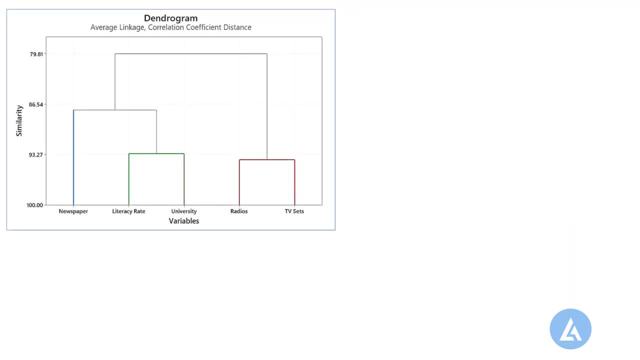 Similar to cluster observations, cluster variables analysis also uses a hierarchical procedure to form the clusters. Variables are grouped that are similar or correlated with each other. At each step, two clusters are formed. The cluster variables analysis is used to determine the number of clusters that are joined, until just one cluster is formed at the final step. 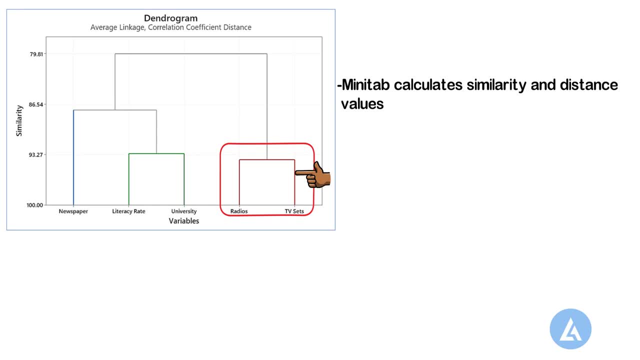 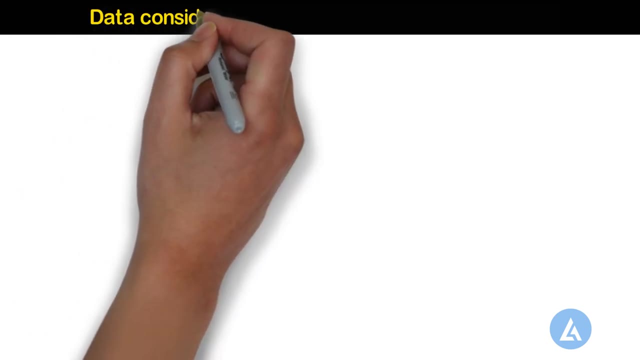 Minitab calculates similarity and distance values for the clusters at each step to help you select the final grouping of variables. You can also display a dendrogram to visualize the clustering results at each step. Data Considerations for Cluster Variables Analysis. To ensure that your 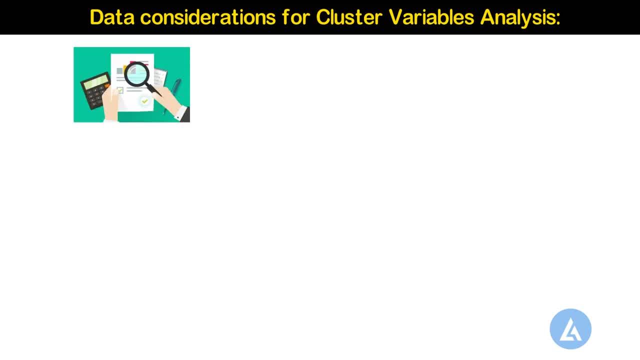 results are valid, consider the following steps. You can also display a dendrogram to visualize the 클� advertises that you have collected in repeated rows of some total number of clusters. Results: The data consideration for cluster variables analysis is the same as that of cluster observation. 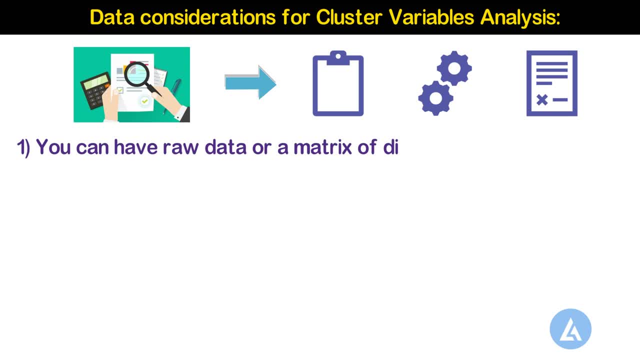 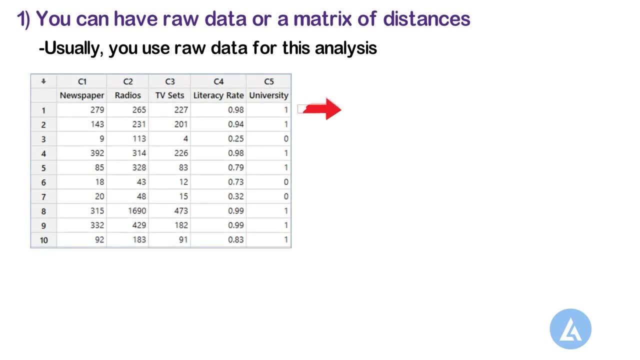 analysis. 1. You can have raw data or a matrix of distances. Usually, you use raw data for this analysis. Each row contains measurements on a single item or subject. You can use the data to evaluate your analysis. You must have two or more numeric columns, with each column representing a different measurement. 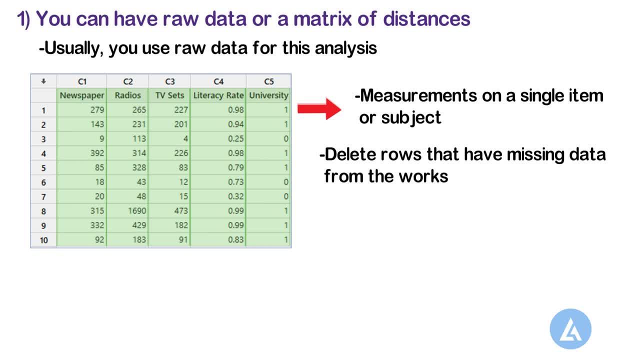 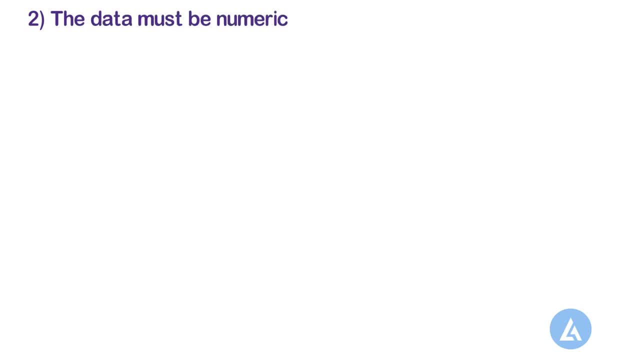 You must delete rows that have missing data from the worksheet before you use this analysis. 2. The data must be numeric To form the clusters. this analysis calculates the distance between observations, which cannot be measured between levels of a categorical variable. 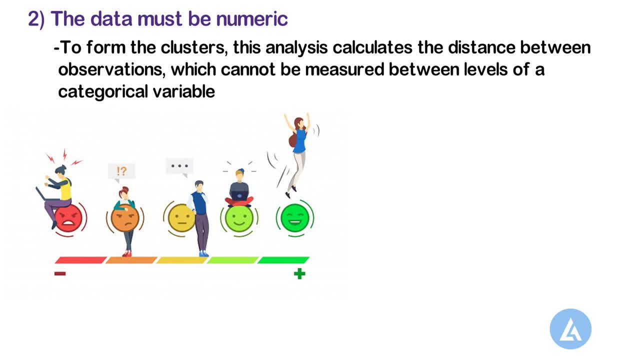 To use a categorical variable in the analysis, you must first convert the text values to a numerical scale. For example, an analyst measures customer satisfaction using the categories very satisfied, satisfied, unsatisfied and very unsatisfied. To perform cluster variables analysis, the analyst records these categories as plus 2, plus 1, minus 1, minus 2.. 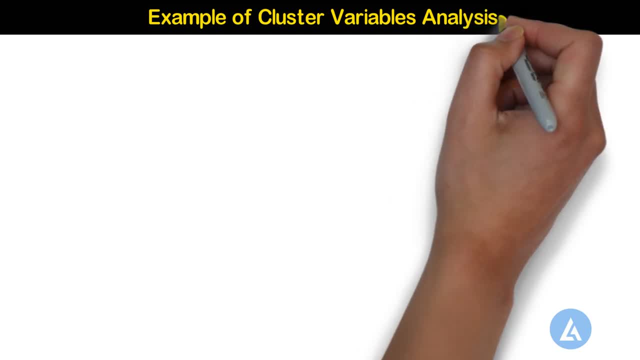 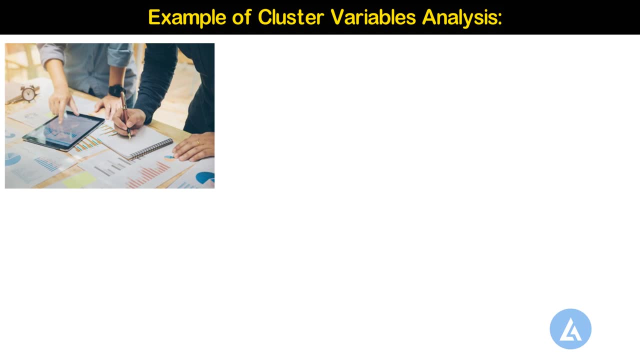 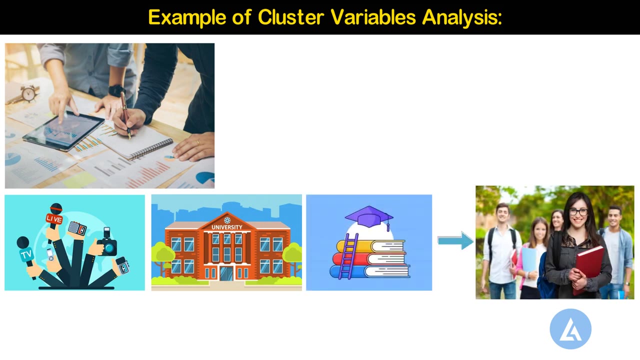 Example of Cluster Variables Analysis. Let's continue with the same example. A social scientist wants to study the effects of the number of media outlets, universities and the literacy rate on the college admissions of the population For 10 cities around the world. the scientist determines the number of newspaper copies, radios and television sets per 1,000 people. 3. The data must be numeric. To form the cluster variables analysis, you must first convert the text values to the categories: very satisfied, unsatisfied, unsatisfied and very unsatisfied. To form the cluster variables analysis, you must first convert the text values to the categories: very satisfied, unsatisfied and very unsatisfied. 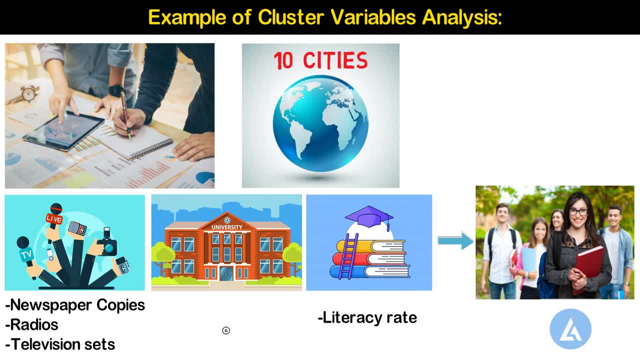 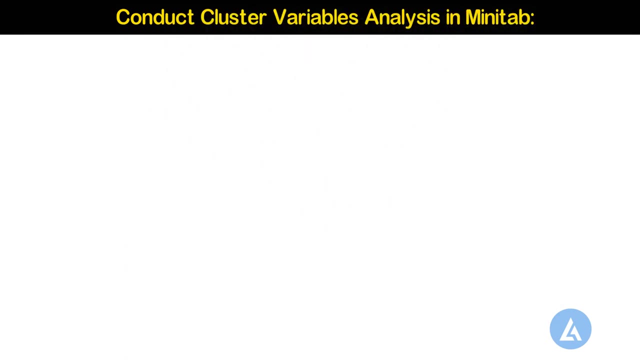 The scientist also records the literacy rate and whether a university is in each city. The scientist wants to reduce the total number of variables by combining variables with similar characteristics. Therefore, a scientist uses cluster variables analysis. Conduct Cluster Variables Analysis in Minitab. To conduct a cluster variables analysis in Minitab, please follow the steps. 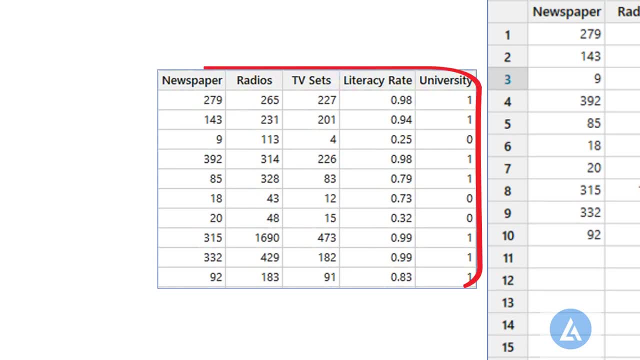 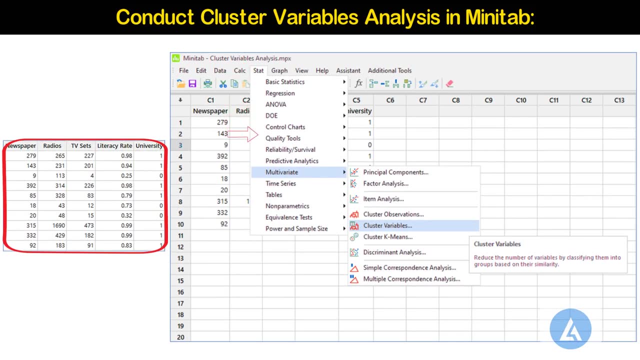 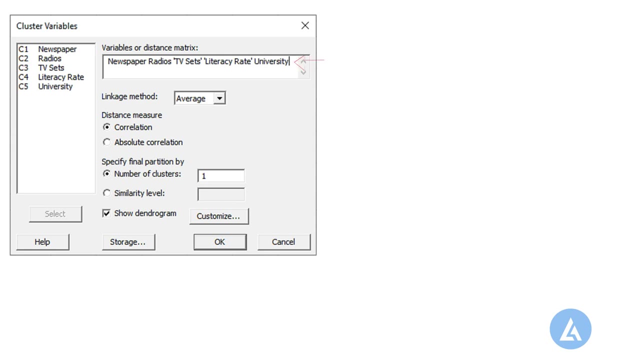 1. Enter or copy the data to the Minitab worksheet as shown in the picture. 2. Select Stat, Multivariate And then cluster variables. 3. In variables or distance matrix, enter newspaper, radios, TV sets, literacy rate and university. 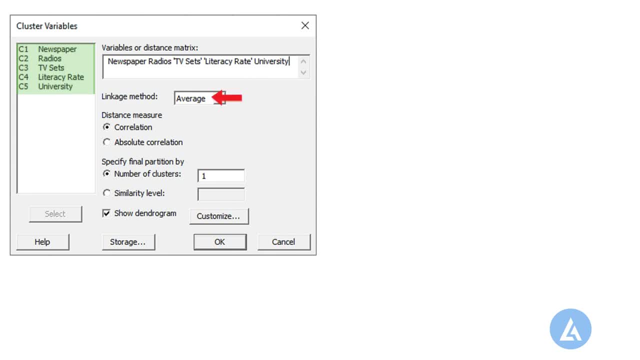 4. From linkage method: select average. 5. From linkage method: select average. The distance between two clusters is the mean distance between a variable in one cluster and a variable in the other cluster, Whereas the single and complete linkage methods are based on single-pair distances. 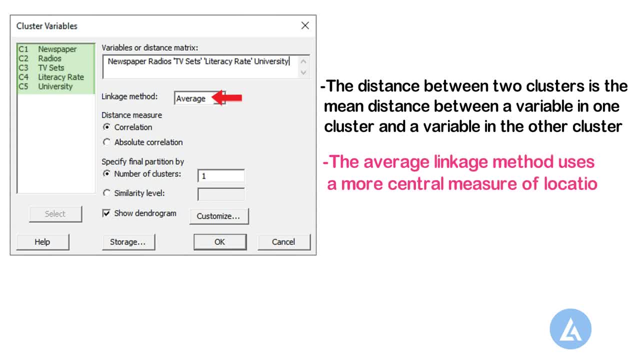 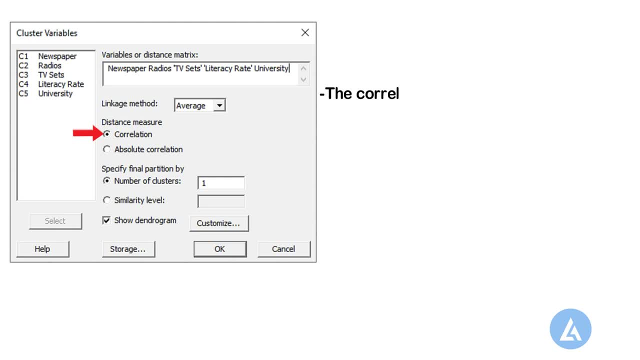 the average linkage method uses a more central measure of location. 5. Under distance measure, select correlation. The correlation method gives distances between 0 and 1 for possible distances On a scale of 1 to 2, consider 1 as a positive correlation and between 1 and 2 as a negative correlation. 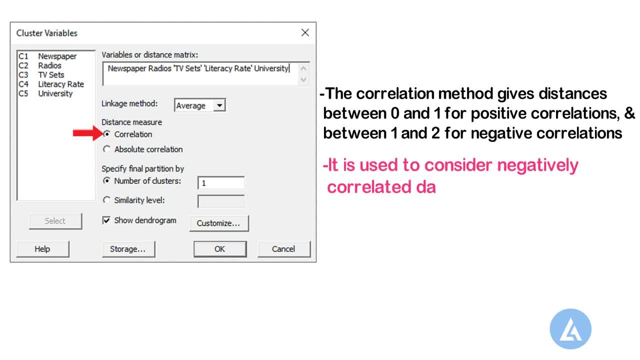 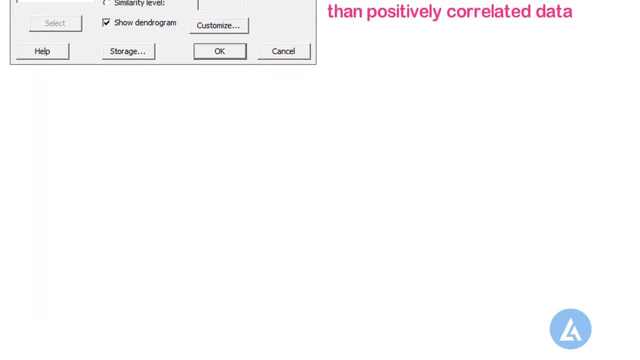 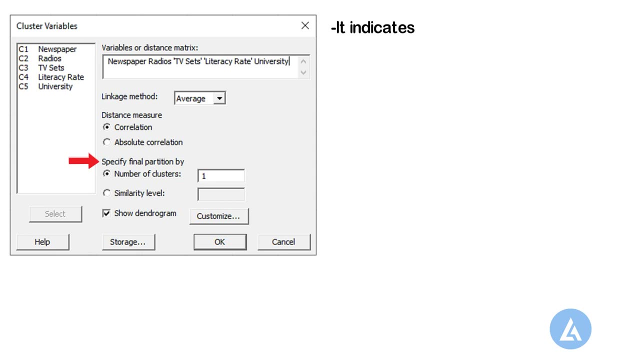 If it makes sense to consider negatively correlated data to be farther apart than positively correlated data, use the correlation method 6.. In Specify Final Partition By. keep all the default settings as it is. It indicates the criteria that you want to use to determine the final groupings. 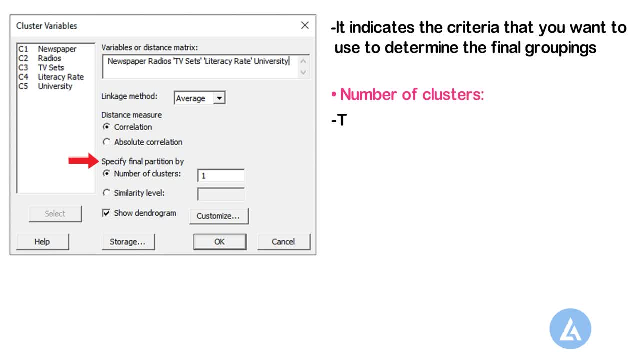 6. Select the option Off number of clusters to enter the number of clusters for the final partition, and select the option of similarity level to enter the similarity level for the clusters in the final partition. 7. Select show dendrogram. Select this option to display a tree diagram that shows how. 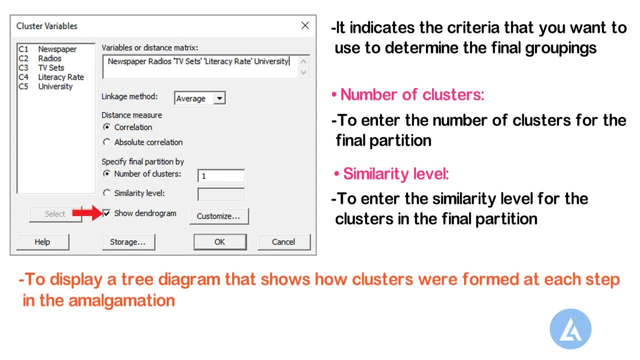 clusters were formed at each step in the amalgamation procedure. The dendrogram allows you to view the similarity or distance values for the clusters at each step And 8.. Click ok in each dialog box to get the results. We will get the results of an analysis in the session window. 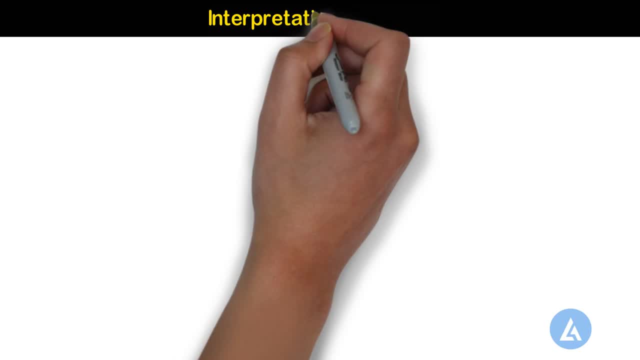 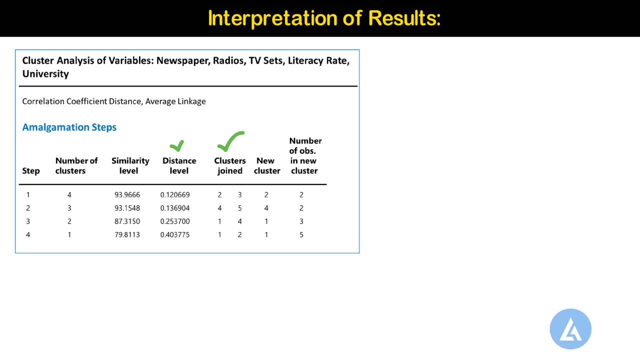 and graph window Interpretation of results. The table shows the clusters that were joined at each step, the distance between the cluster and the similarity of the clusters. The similarity levels are shown in the dendrogram. The similarity levels are shown in the dendrogram: The similarity. 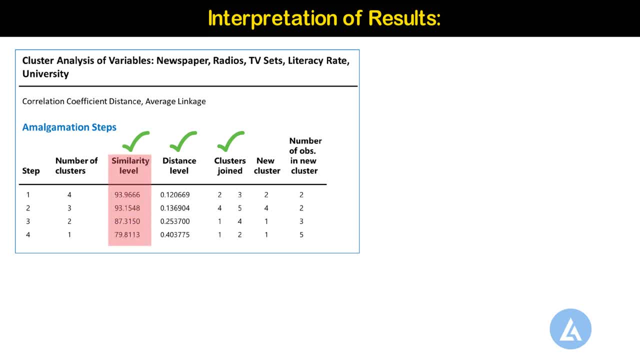 level decreases slightly from step 1, 93.9666, to step 2, 93.1548, then decreases suddenly in step 3, 87.3150, when the number of clusters changes from 3 to 2.. The distance between the joined